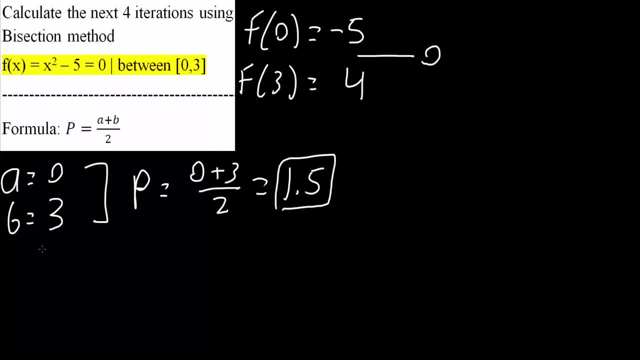 by two. But the second iteration, and the third and fourth, Involves using a and b, And I will explain why. So now we want to get the second iteration. So in order to do so, we need to determine the function of p. So p is one point five. 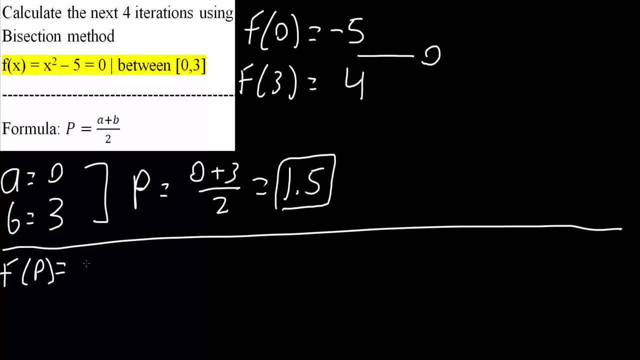 We will plug in one point five back here And see what would happen. And so when we plug it in, we get one point five squared minus five, And that is going to equal negative two point seven five. Now this is important: We get a negative number. 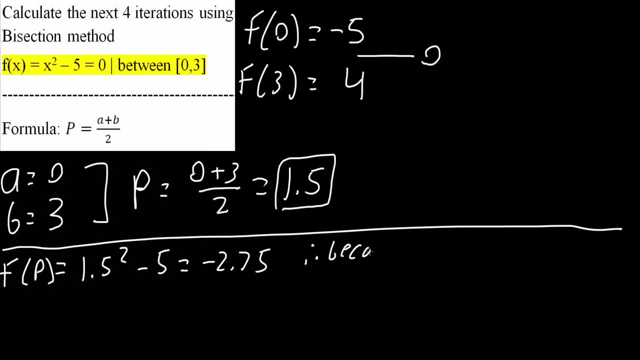 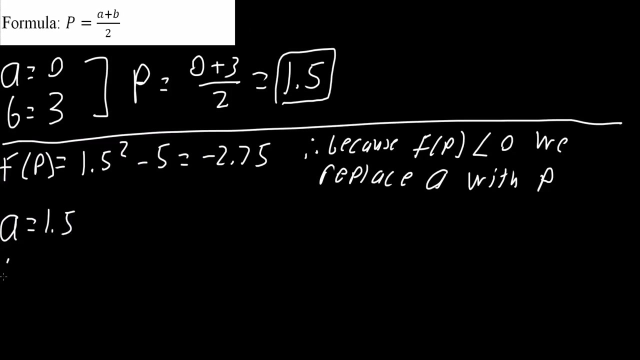 And this is a rule here, Because f of p is less than zero, We replace a with p. This is an important rule, And so now we have: a is equal to one point five and b is equal to three. b remains the same. 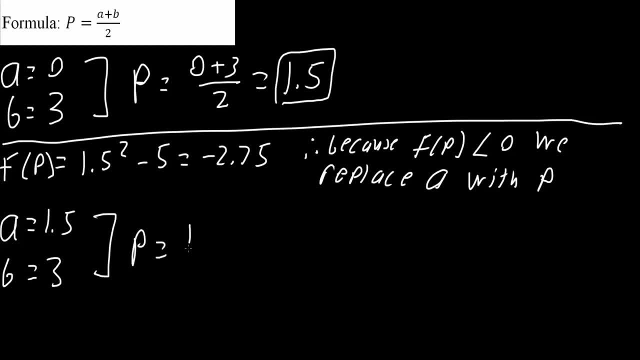 So P is equal to 1.5 plus 3 divided by 2.. So that would equal 2.25.. This right here is the second iteration, but we want to get four iterations, so we need to do it two more times. 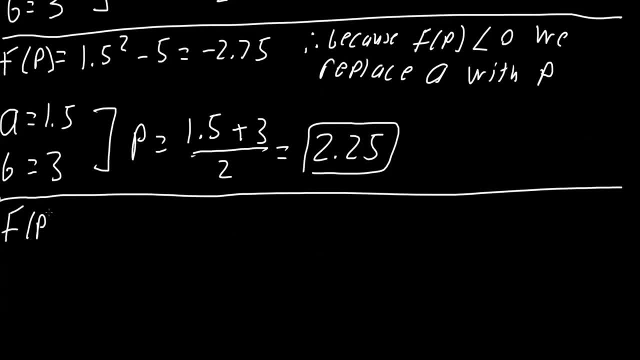 And now we'll do the same idea. We get F of P. In this case P is 2.25.. So we say equal 2.25 squared minus 5, and that would give us a positive 0.0625.. 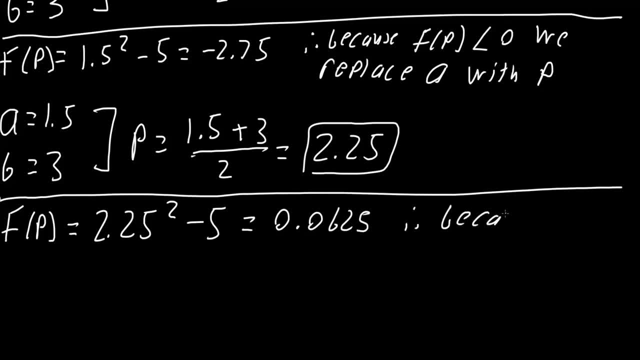 Now this is another rule. Because F of P is greater than 0, we replace B with P, Another rule. So now A Remains the same, A is here is 1.5.. A will remain the same And B will change from 3 to 2.25. 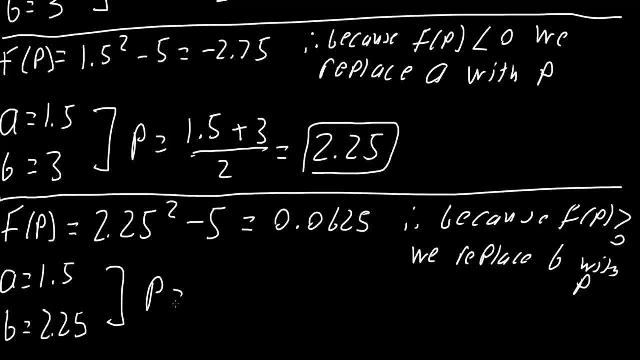 And so now it's the same idea, getting P. P is equal to 1.5 plus 2.25 divided by 2., And we would ultimately get 1.875.. And we can box in this answer. Now we'll do it one more time. 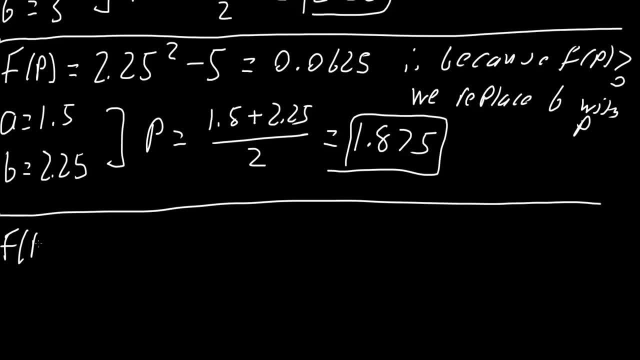 So same idea. We get F of P. In this case P is 1.875.. 1.875 squared minus 5. And we would get negative 1.484.. And because it is negative, we replace A with P. 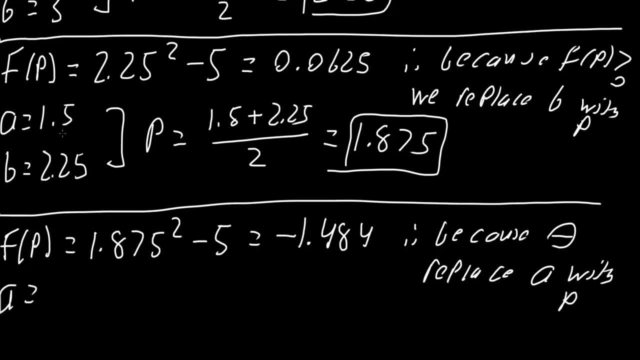 Okay, So now A will go from 1.5 to 1.875, and B will remain the same: 2.25.. And in doing so, P will equal 1.875 plus 2.25 divided by 2, and we would get 2.063. 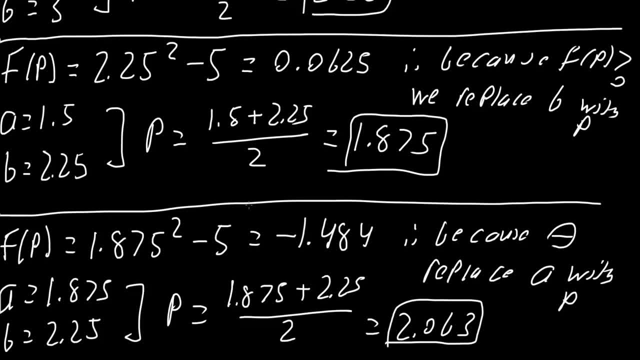 So this is the fourth iteration. Ideally we would not stop here. We would continue until A and B are very, very close to each other. So originally A was 0 and B was 3.. But as we keep on doing this, A and B will become closer and closer together. 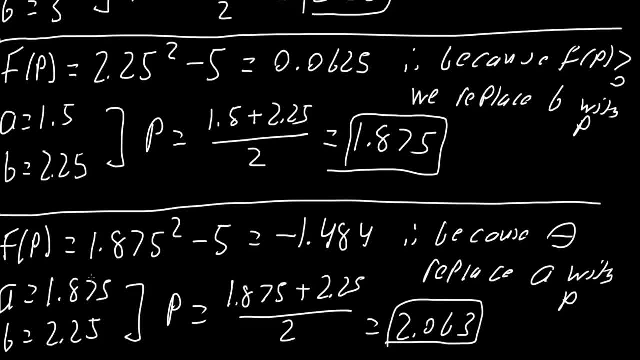 So you know, if we use a computer algebra system, you know it would automatically keep on doing this iteration for us until essentially A and B are the same number. But in an exam, if it asks us to solve by hand, this is what we would do. 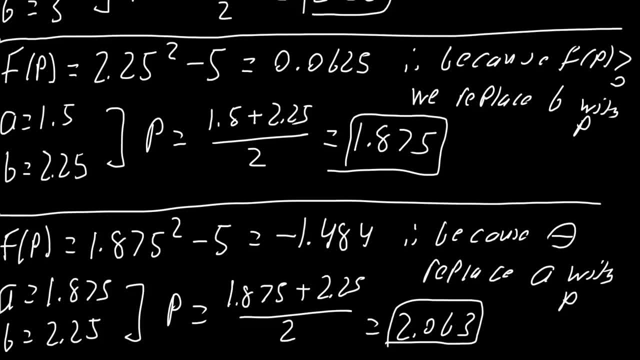 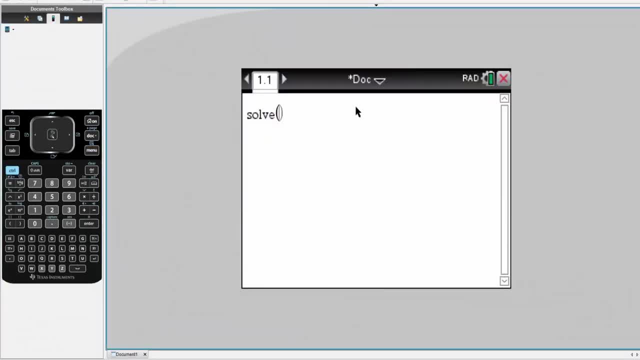 So just to show that this answer is pretty, Pretty good, I will solve this question using a TI Inspire. So let's do that. So menu algebra solve. I had x squared minus 5 is equal to 0, and we want to solve for x. 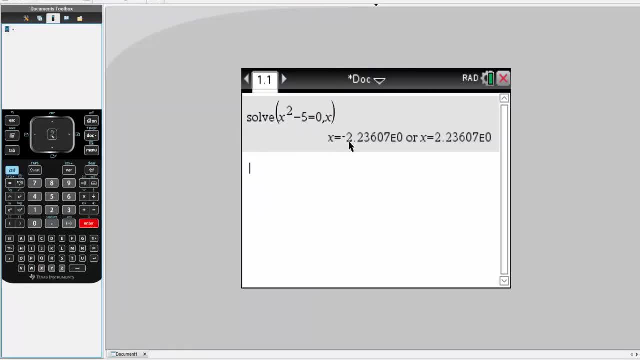 I hit control enter. So one number for x would be negative- 2.23.. The other would be positive, 2.236.. The answer that we got was 2.0.. So after four iterations we're still a bit off. 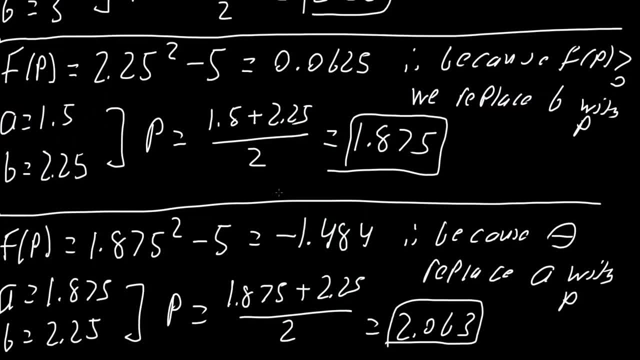 But had we kept on continuing and continuing, we would have been closer and closer to our answer. But now you may ask: why did we only get a positive answer and not the negative one? And so let me explain that. So we want it from between 0 and 3..